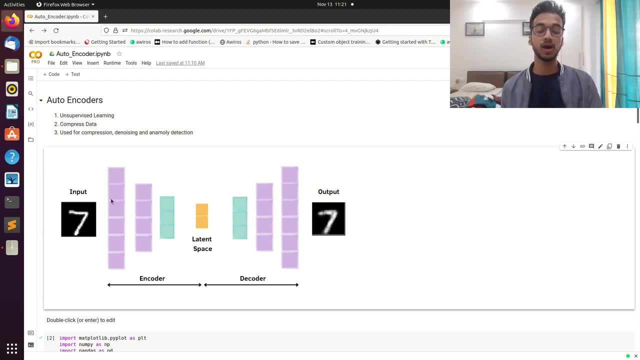 what's called as the encoder, And so, as the image is being passed from one layer to the other, it's constantly getting reduced in dimension, and this yellow and this orange box that you're seeing is called as the Latin space. It's basically the compressed form. 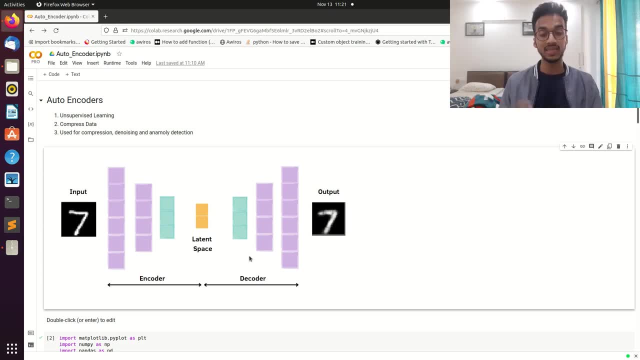 of that same image. And then we have a decoder which takes back that compressed data right and reconstructs back the original image from it. Now, when you look at this diagram it might seem pretty useless, because you're taking the same image, compressing it and then 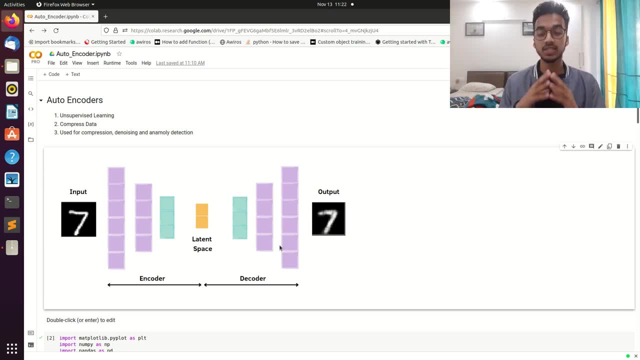 decompressing it to get back the same image. But the reason it is so useful is that if you can take an image, compress it down to a smaller dimension. let's say you take an input image of 28 cross 28,, which is 784 pixels. you compress it down to, let's say, only 64. pixels. After compressing it to 64 pixels, you can compress it down to, let's say, 64 pixels. After compressing it to 64 pixels, you can compress it down to, let's say, only 64 pixels. After compressing it to 64 pixels, you can compress it down to, let's say, only 64 pixels. 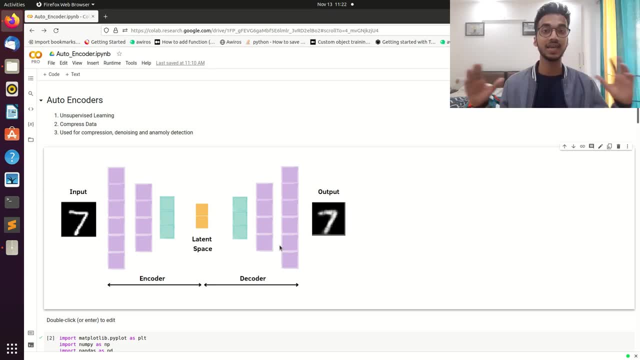 After compressing it to 64 pixels. you can compress it down to, let's say, only 64 pixels. If you're able to reconstruct it back to the original image, that means that the only most important information of that image is conveyed in those 64 pixels that you were able to compress. 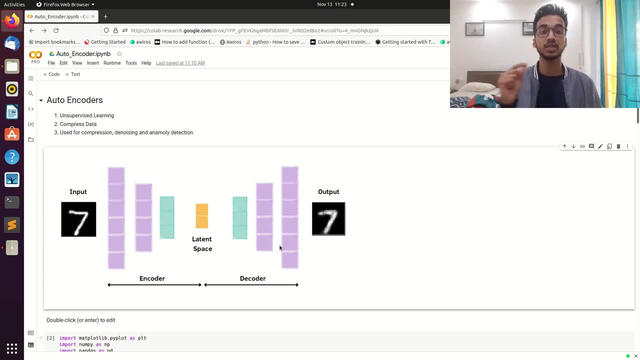 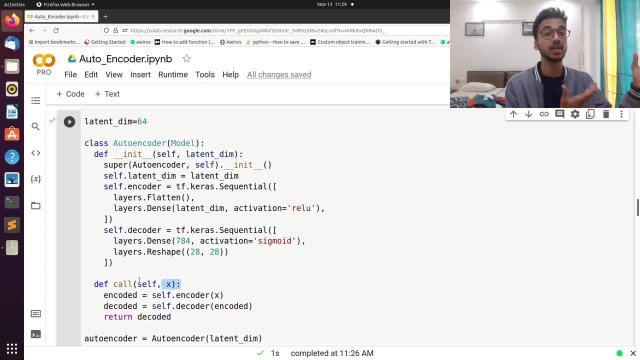 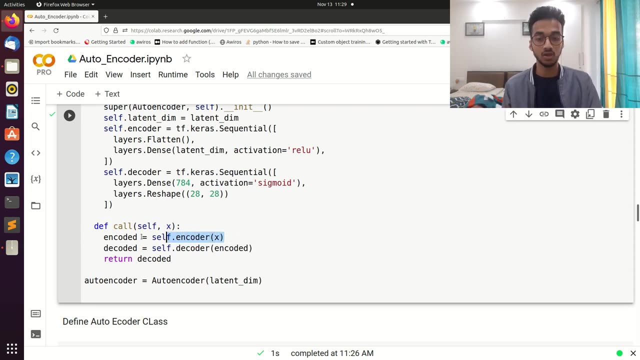 we still not have told the model that hey, when you get an input, pass it to the encoder first, then pass it to the decoder. right now it does not know all of that. so that is what happens in the call function. we first take an input- image x- we pass it to the encoder right and save it as encoded. 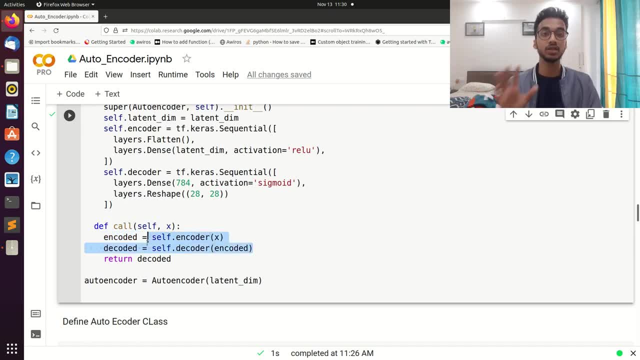 and then we take this encoded image and then pass it to the decoder. finally, what the output of the decoder was, that is going to be returned by this class, right? so this was just the definition of the class over here. we're going to call it and we simply have to provide the latin dimension. 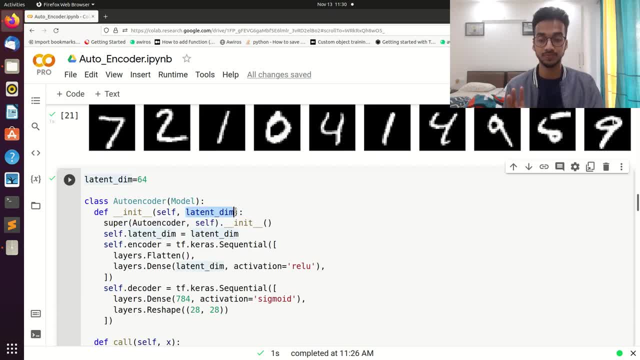 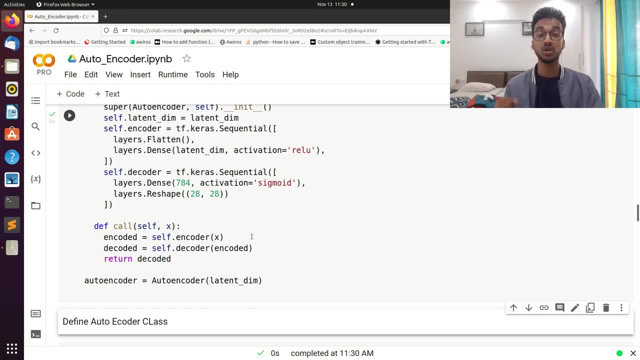 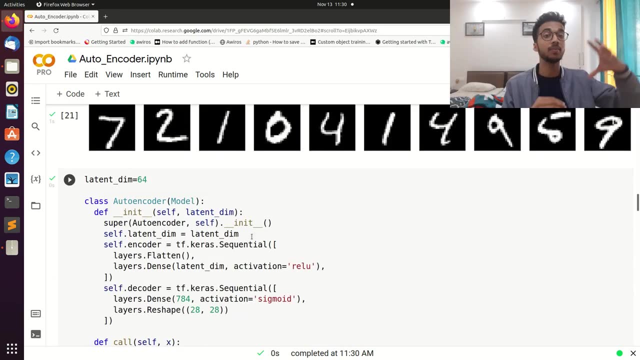 because that is only the input parameter we had defined over here. so our auto encoder is class, is all built and ready. now we have to train that model right now. why do we need to train it? because we take an input image, we compress it, decompress it back to the original image, right, but in the first. 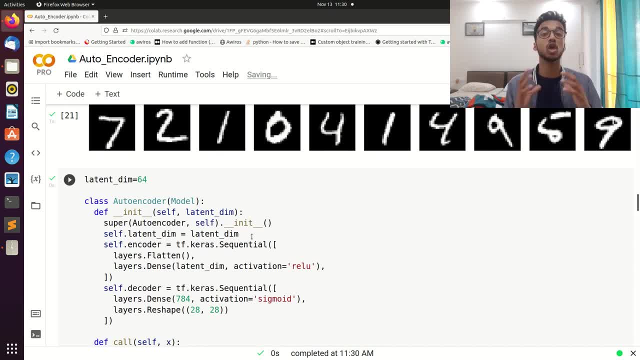 iteration. it's not going to do a very good job. it's not going to be able to reconnect, constructed to the exact same input image, so there's going to be a difference between what the input image was and what it was able to get as the output. so the difference between these two 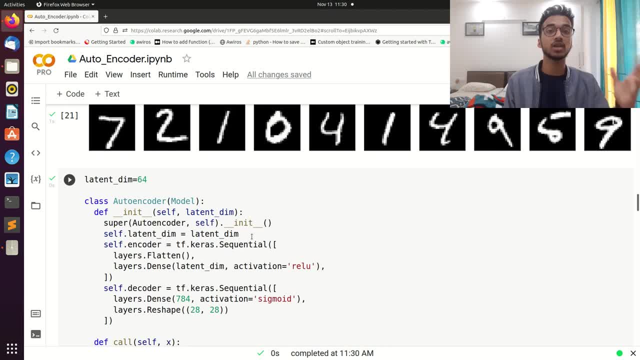 the actual output and the reconstructed output, as you can call it, will be the loss, and the goal with training is that with various iterations it will be able to minimize the loss. so whenever you compress it and decompress it, you will get the exact same input image as before. 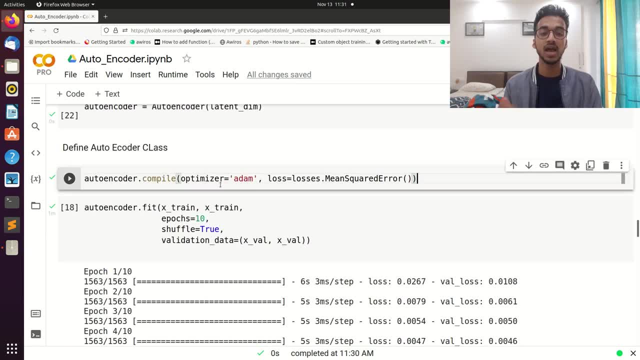 that we first compile the model using the atom optimizer and we use simply the mean squared error, which will simply check the mean squared error of of pixel difference between the actual output and the reconstructed output by the decoder right. so over here we call the fit function to train the 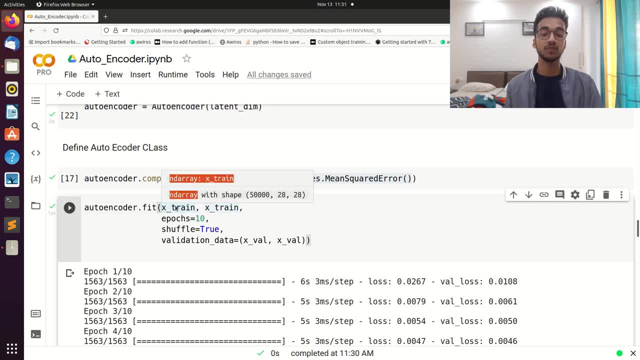 model. the argument for the fit function is going to be x train, which is the input to the model, and the output is also going to be same as the input, because the entire goal of the model is that it has to construct the same image as the input. so the input and output are going to be same in this. 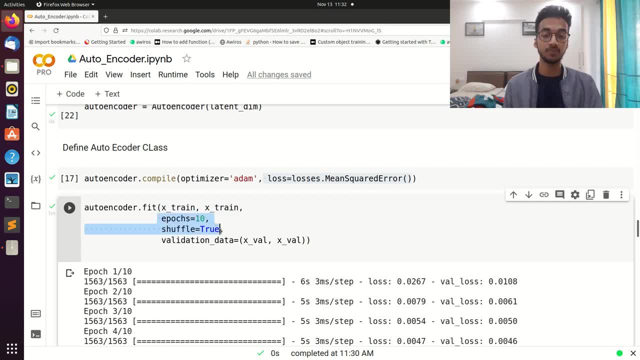 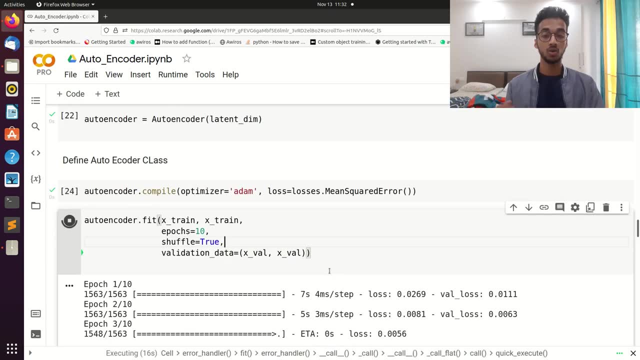 case, so be careful when you're writing this code. we run it over 10 epochs and we provide the validation data over here, and once i run this line, training will start. it will probably take a minute. once it has been trained, you're going to be able to see the output and i'm also going to show you. 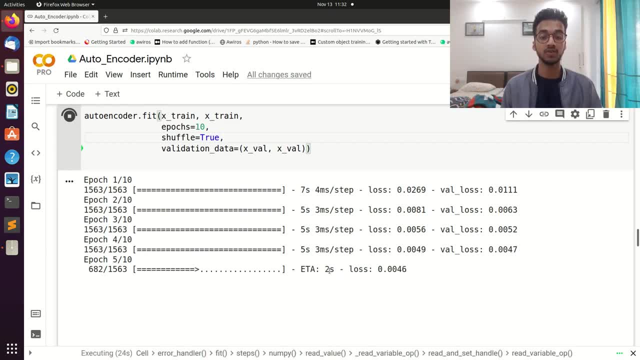 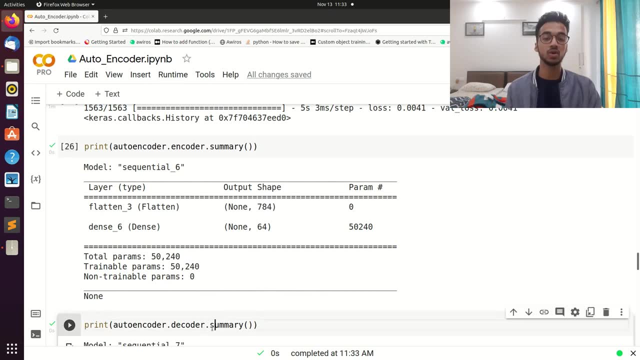 the architecture as well for this exact code that we have written. so now i'm printing the summary of the encoder and i'm also going to print the summary of the decoder as well. you can see the original input of 28 cross 28 was converted into 784 pixels by the flattened layer. 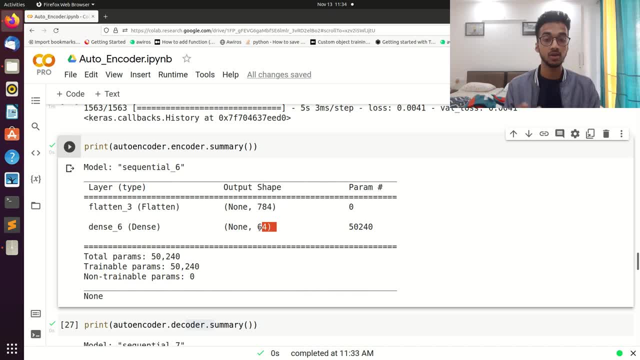 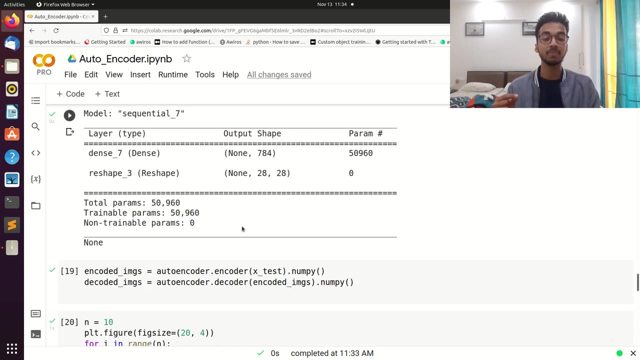 which was then converted into 64 layers by the dense layer, which means the input information of 28 plus 28 is now confined into 64 pixels. these are the pixels which contain all the information. now the decoder takes the 64 pixels and then again maps it back to 784. 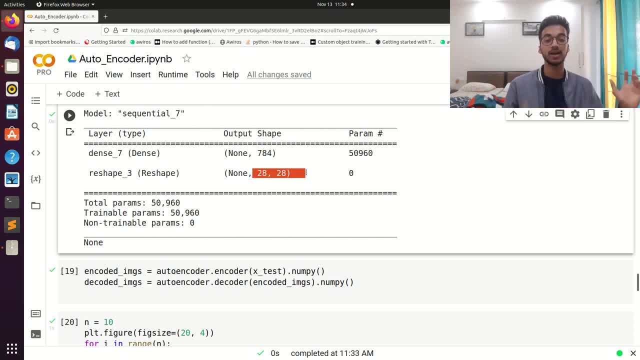 and then 28 plus 28 and we get the original image back to test this model a little bit in practice to see how it works. we're gonna take some test images over here, we're gonna pass it to the encoder and save it as encoded images. then we take these encoded images and pass it to the. 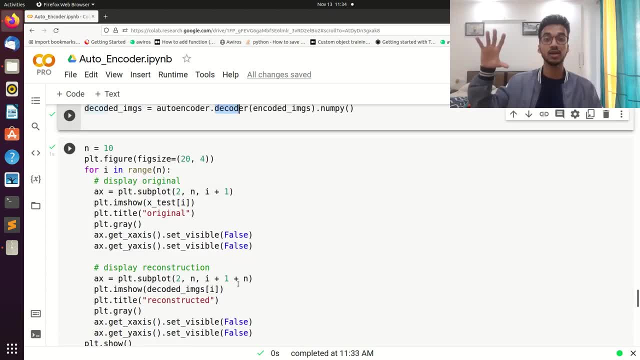 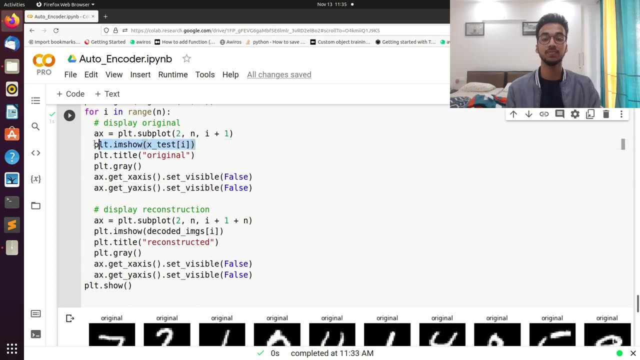 decoder. again over here i'm gonna plot what the actual images were and what the reconstructed images were by the decoder. so again, i iterate through 10 images and i'm going to create some subplots and this is very basic matplot visualization. basically, i'm printing the x test initially, then i and then i.